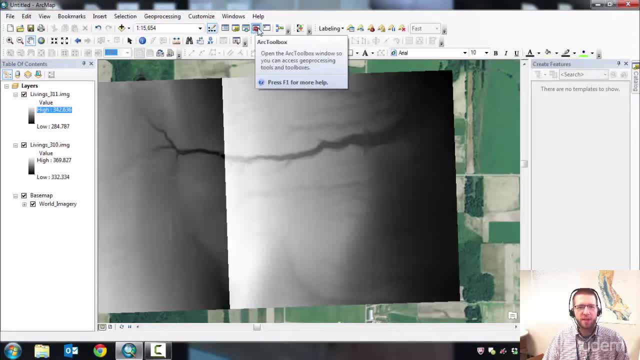 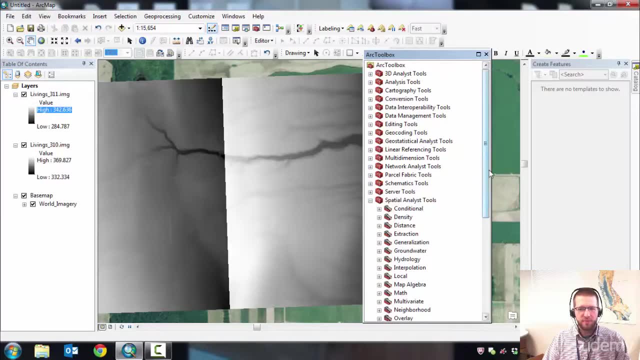 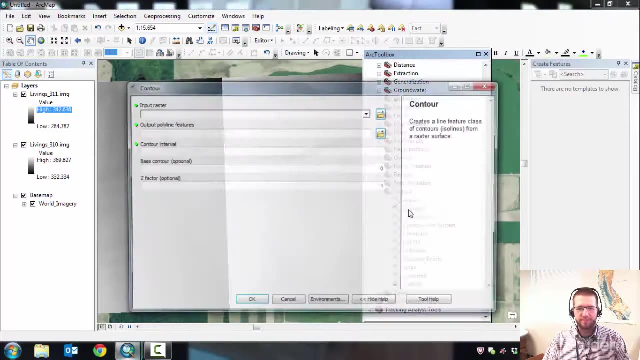 Go to Spatial Analyst, which you can find in the Arc Toolbox- That's this little red toolbox button. Scroll down to Spatial Analyst Tools And inside there you're looking for the Surface Tools. Inside Surface Tools. you want Contour? Okay, it'll ask for an input raster. Let's just do 311.. 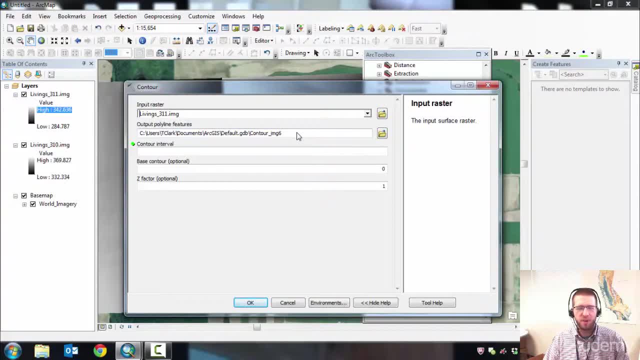 It's going to put Polyline features in. It's looking for a geodatabase, so I'm just going to use my default geodatabase. I use that for lots of stuff. Contour interval: this is the spacing between the contours that you want. 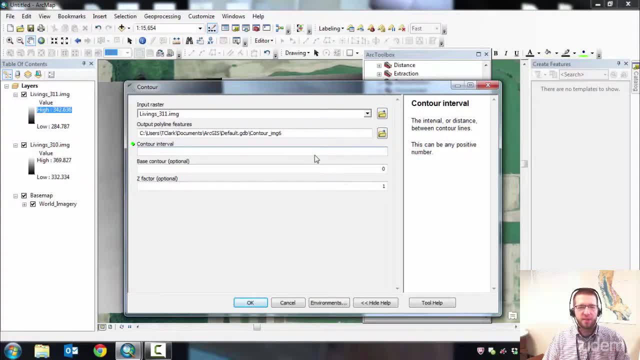 And we're going to convert it to English So you can put in your English contour interval. here It's going to be, let's say, 10 feet for us. Okay, Base contour. if you want contours every 10 feet on the 10s, just use 0.. 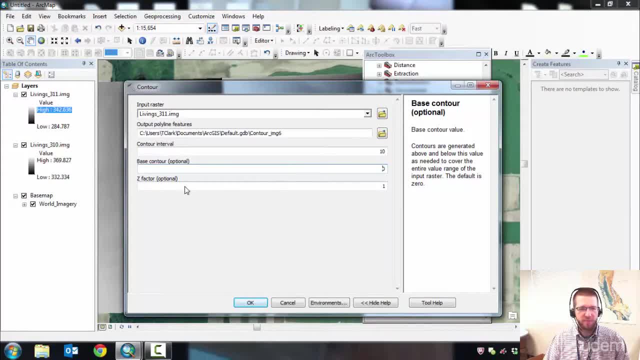 And that'll be the best bet for you. Z factor. this is going to be that conversion factor from English to metric. So, since we're going from metric to English, I like to remember it as there's. you know, English feet are smaller units than metric. 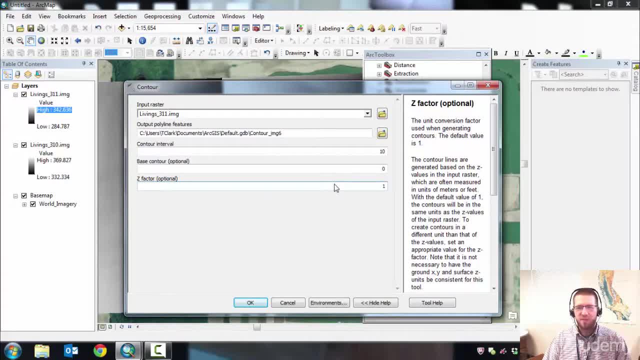 So if I have 100 meters, I'm going to have much more feet And that means I'm going to multiply by a number bigger than 1.. And fortunately those conversion factors are right in the help over here. If you could just scroll down. 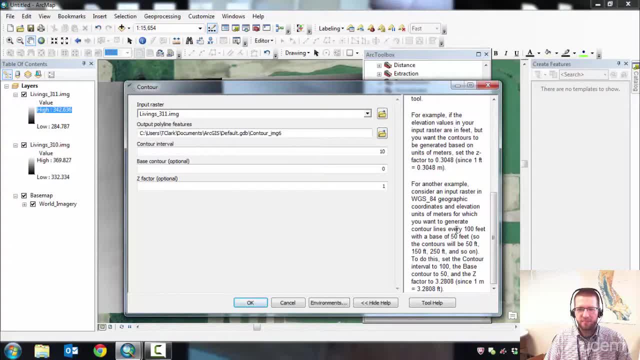 And it's so. this one is a second one. For another example, consider input raster in WGS 84.. Elevation uses meters. You want to generate contour lines every 100 feet with a base of 50.. Okay, we're doing a base of 0.. 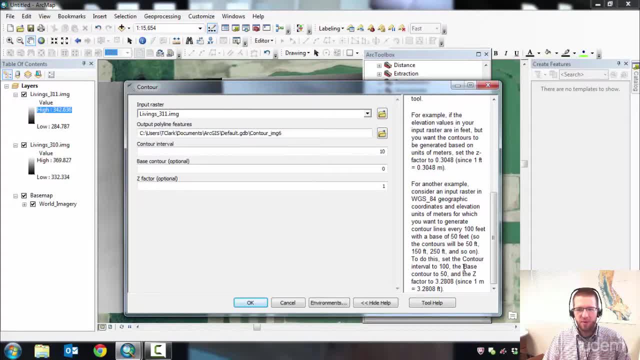 And so on. Set the contour interval, the base contour and the z factor to 3.2808.. So we're just going to use that bit of information: 3.2808.. Hit okay, And then it'll chug along. 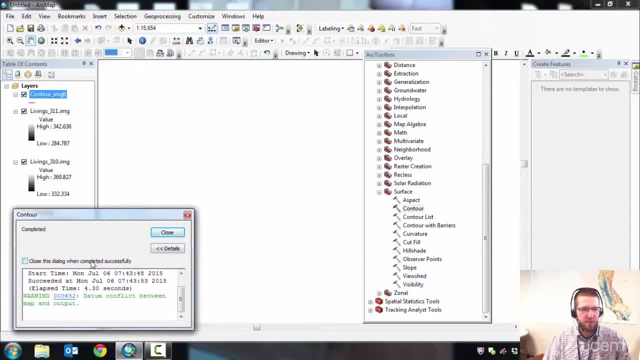 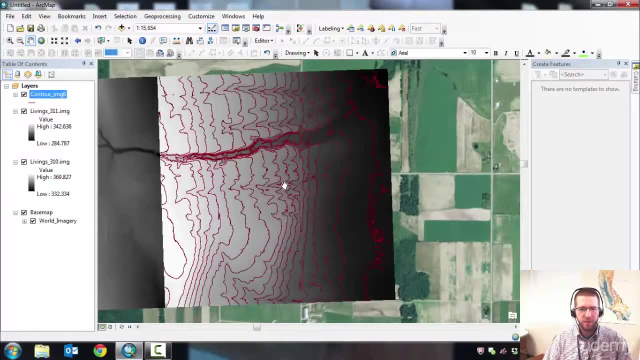 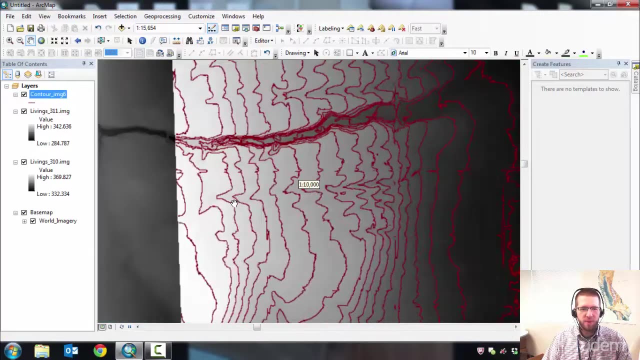 I have it on no background geoprocessing, so we'll see how it goes. Close it, Close that, And then you have your contours, So now you can use this data To generate your watershed. Definitely want to note, though: When you display the lidar contours, they're very jagged. 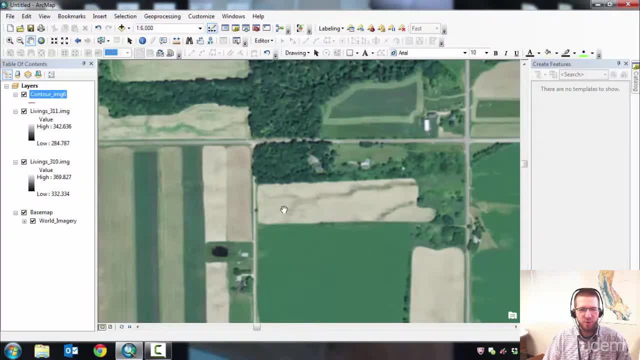 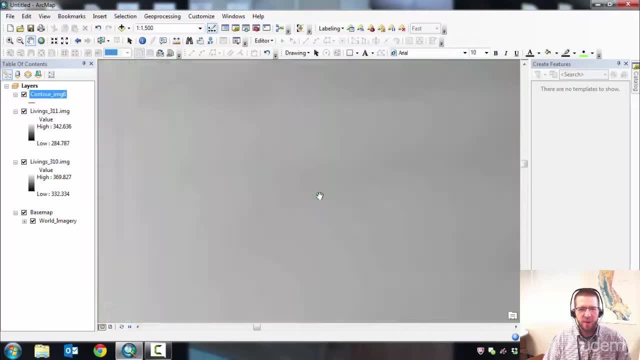 That's because the data is very dense and it hasn't been smoothed by computers yet, Although it can be. You can do that to get a better map view, And I mention this because one of the methods that we typically use for hydrology is: 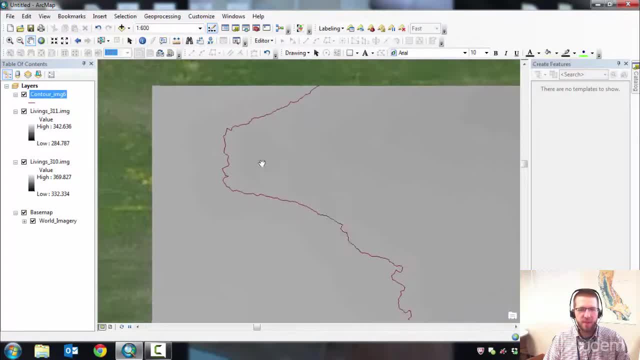 The average slope of the watershed to get time of concentration. And one of the ways we do average slope is the contour length method And if you're using lidar data with really jagged contours, If you try and do contour length method in GIS where you just add up the lengths of the features. 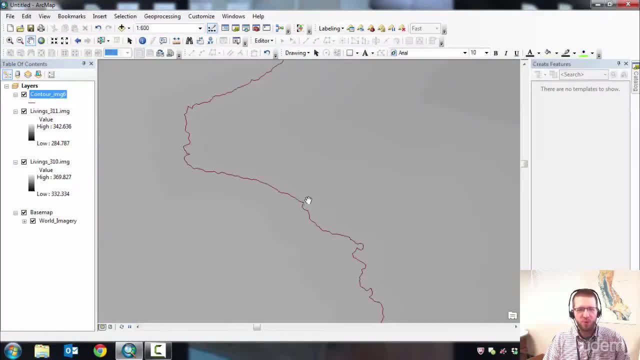 It's not going to work quite right because the contours will be too long. Okay, The contour length method is meant to be used by heat And methods on USGS contours, Not using a computer on lidar contours. So just bear that in mind. 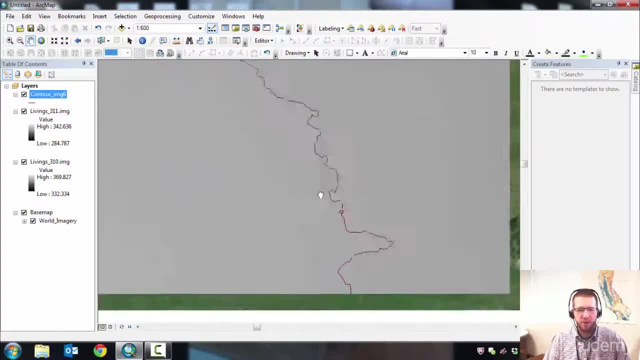 We're going to look at some other ways to do the average watershed slope later on too, All right. So if you have ArcMap with Spatial Analyst, Check and see if there's lidar available in your area. Download some and try and display those contours. 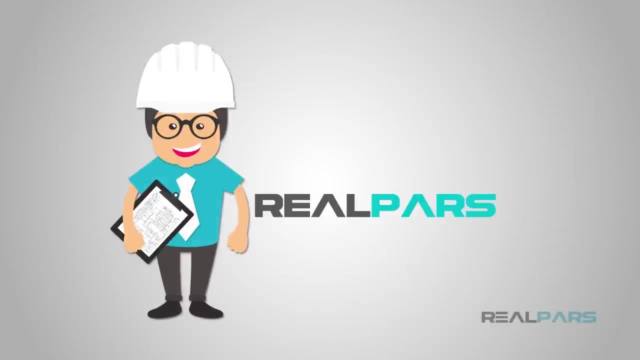 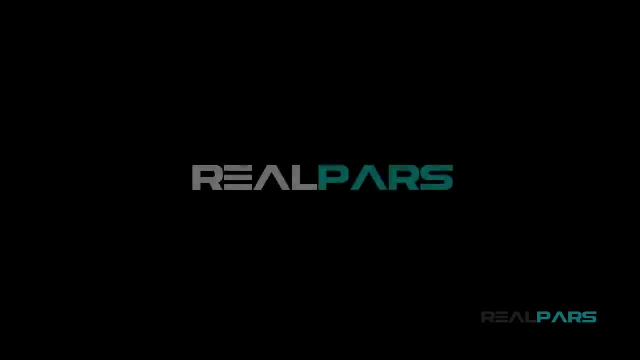 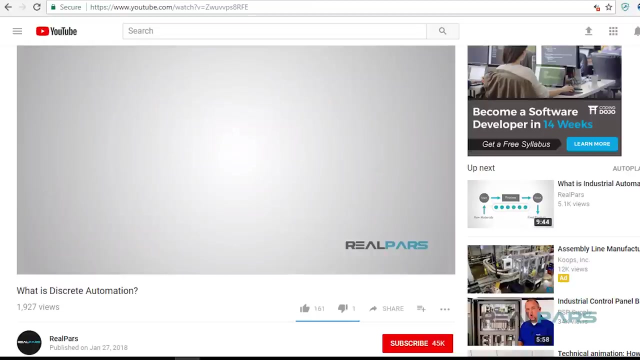 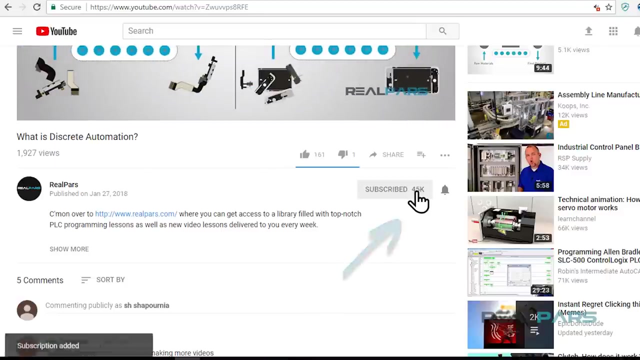 Welcome to another informative video from RealPars. Today you'll learn all about HMIs. Before starting this video, I want to remind you that if you're new to the RealPars channel here on YouTube, be sure to click the subscribe button below.